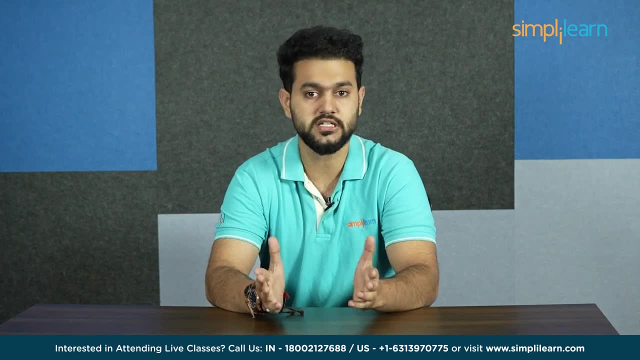 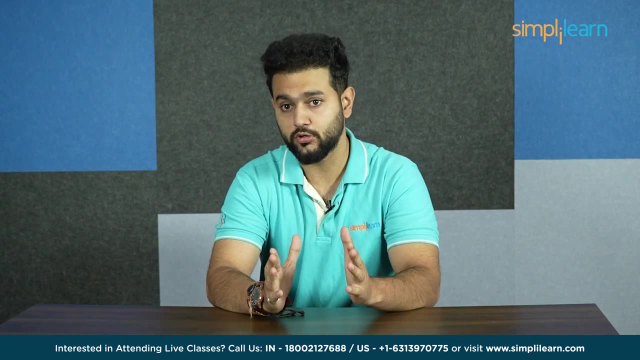 help us process data and use it for the things like machine learning, From managing and processing data to conducting sophisticated machine learning analysis, these technologies play an important role in using the immense power of data. They are like the tools in a data scientist's toolbox. 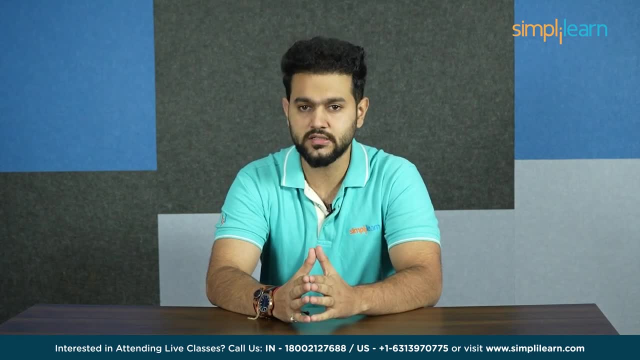 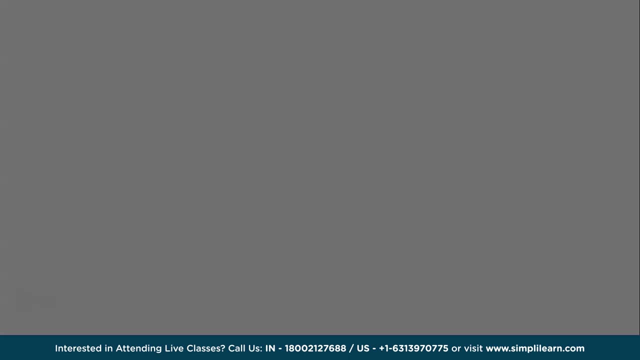 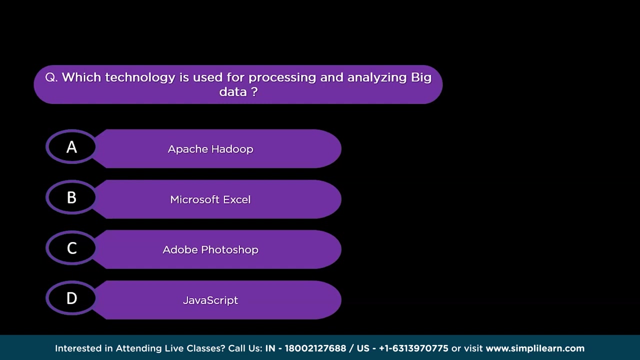 enabling businesses to make informed decisions, optimize operations and gain a competitive edge. So let's get started with this video, But before we begin, let me ask you a quick question. So which technology is commonly used for processing and analyzing big data? Option A is Apache Hadoop. 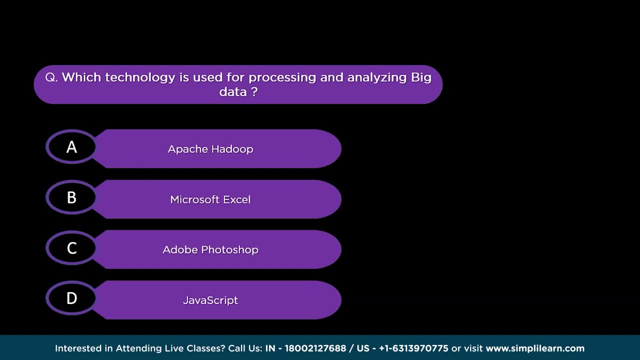 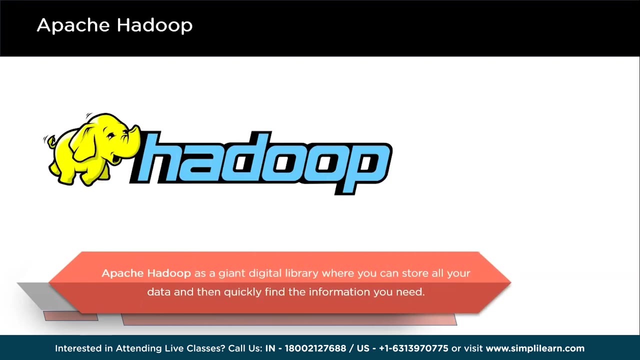 Option B is Microsoft Excel, Option C is Adobe Photoshop and Option D is JavaScript. Now you can pause this video and answer in the comment section below. So let's start exploring these important technologies. First technology on the list is Apache Hadoop. Apache Hadoop is like a superhero of the big data world. It is an 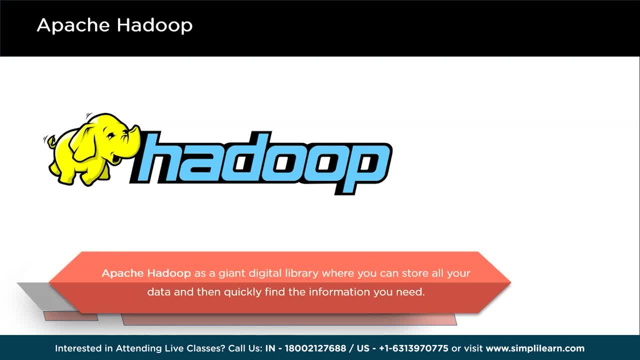 amazing open-source tool that's been at the heart of big data revolution. Think of it as a magical framework that's specially designed to handle and make sense of incredibly huge piles of data, all while using a bunch of tools. So let's get started. So let's get started. So let's get started, So let's. 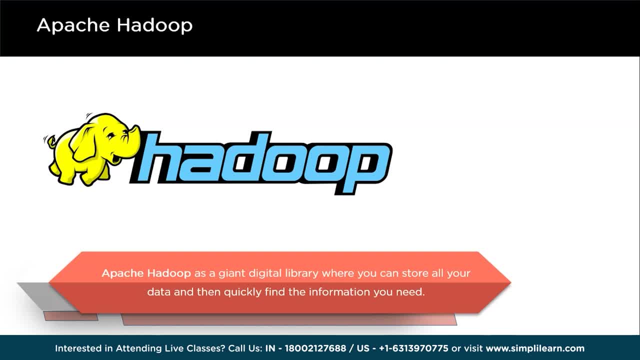 dig right into theай. we have a bunch of regular computers Now. the secret source of Hadoop is its two main parts, that is, Hadoop Distributed File Systems, ADFS and MapReduce, HDFS, along with mobile dataUh like a super organized, the librarian that keeps all. 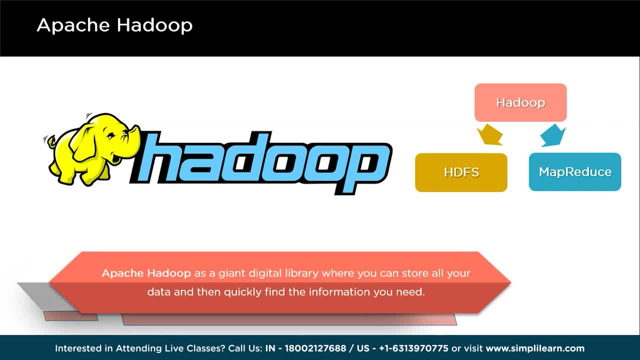 your data neatly in order, And MapReduce is like a team of super fast workers who can process these data lightning quick. The cool thing about Hadoop is that it can work with many regular everyday computers, making it super flexible and cost-effective. you will notice the level ofit. 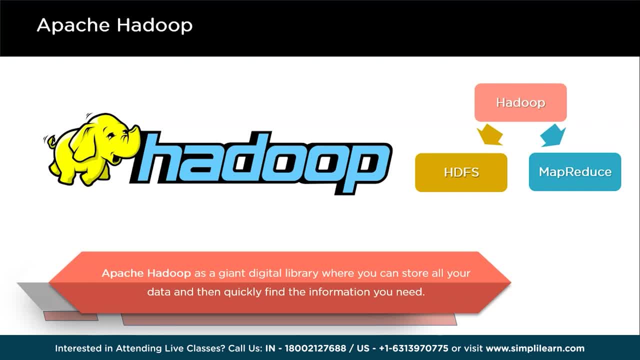 you will notice the level ofit. don't need any fancy, expensive hardware, etc. Hadoop can take your data and spread it out across many computers like a big puzzle. this way it's stored safely and processed super fast because all these computers can work on it together. this 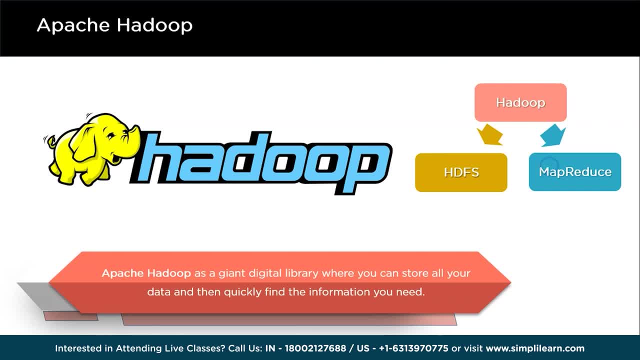 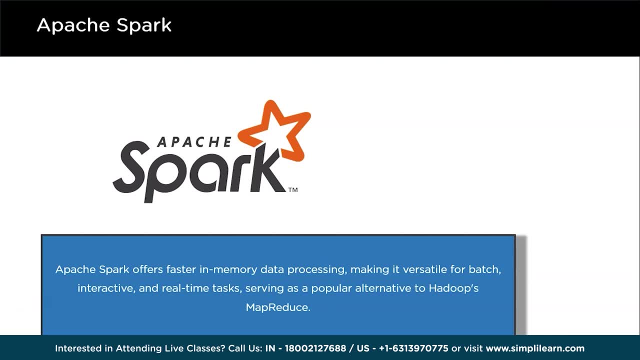 was about Apache Hadoop. now second on the list we have is Apache spark. the Apache spark is a popular and efficient tool that can be used instead of Hadoop's MapReduce. it has a special feature called in-memory processing, which means it can work with data faster. this makes it a great choice for people who work. 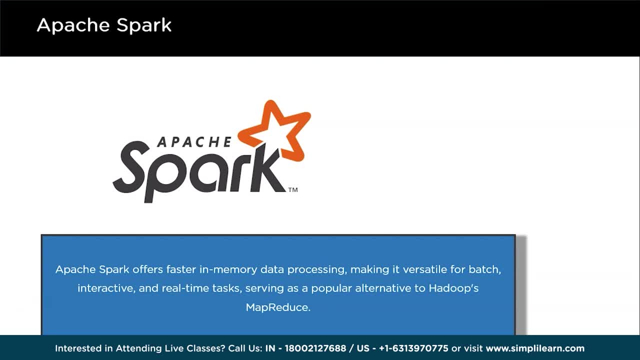 with data, like engineers and analysts. what's cool about spark is that it can do a lot of different things. it can handle batch processing, interactive queries and real-time data streaming, and even process data as its chameleon. this makes it a flexible and powerful tool. so, in summary, Apache spark is fast and 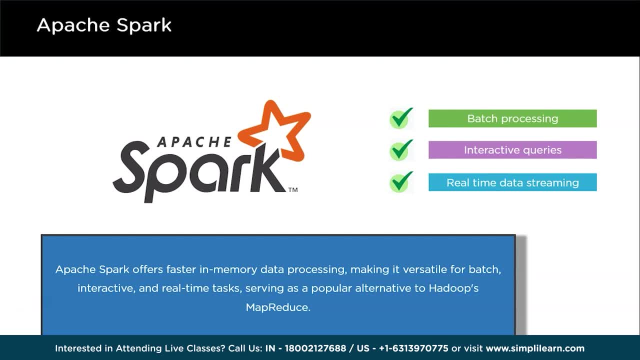 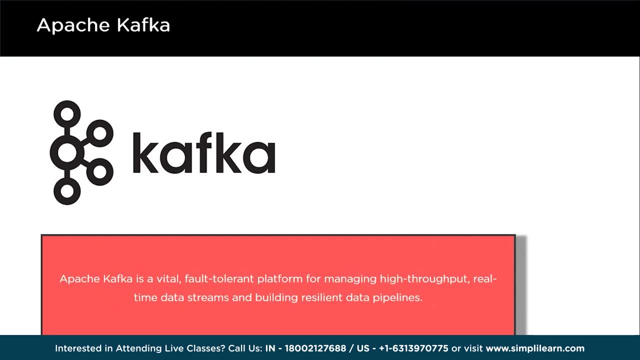 versatile tool that's great for people who work with data. it can do a lot of different things and is preferred choice for many professionals. next we have have is Apache Kafka. Apache Kafka is a super smart messenger for data. It's designed to handle lots of information flying around in real time. Imagine you have a huge amount of data that needs to be. 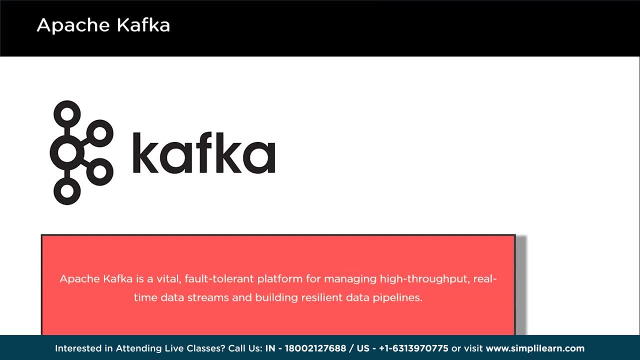 sent from one place to another quickly and safely. That's where Kafka comes in. Think of it as a super highway for data, where information can flow smoothly and reliably. It's like having a special mail system that never loses your letters or packages, no matter how much you send. Kafka is 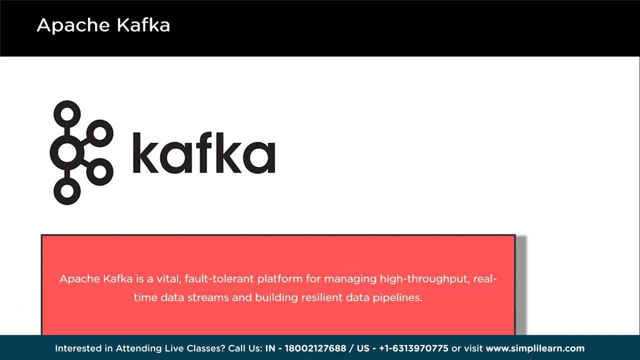 super important because it helps businesses and applications keep up with the latest information. It's like having a news feed that never stops updating, So you always know what's happening right now. One of the cool things about Kafka is that it can handle a lot of data at once. 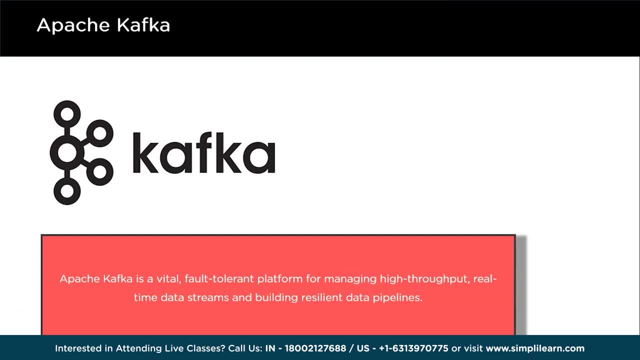 and it's really good at making sure none of that data gets lost along the way. So if you're building a system that needs to stay update in real time, Kafka is a key tool to have in your toolkit. Next big data technology in 2024 is Apache Hive. Apache Hive is a helpful tool that 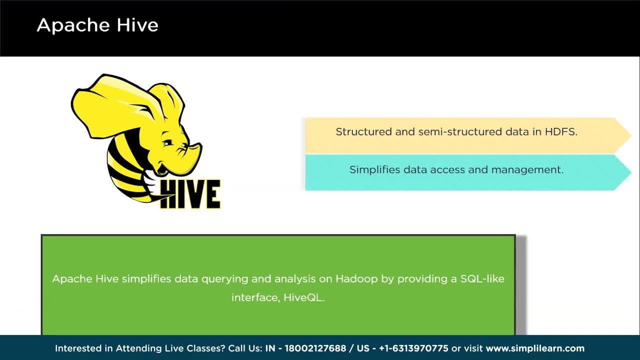 makes it easy for you to handle a lot of data at once. It's a tool that you can use to connect people, to analyze and query data stored in Hadoop. It does this by providing a user-friendly interface that looks a lot like SQL called HiveQL. This means that even if you are not a tech expert, 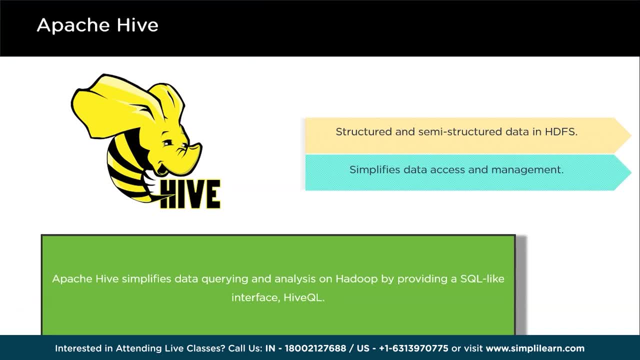 you can still use Hive to work with data in Hadoop. Hive takes the queries you write and turns them into tasks that can be processed by Hadoop's MapReduce or Apache Tests. These are just fancy terms for the behind-the-scenes operations that happen in Hadoop to process. 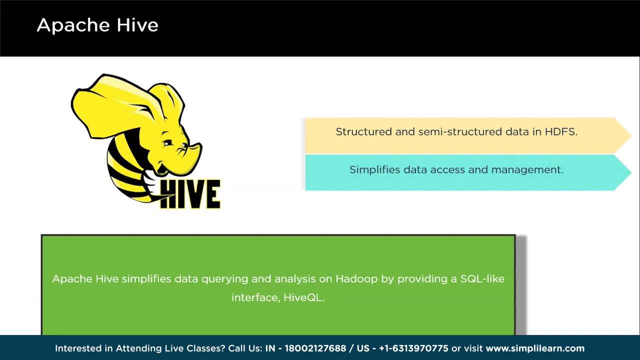 and analyze data, So you don't have to worry about the nitty-gritty details. Hive takes care it for you Here. the Hadoop itself can store all sorts of data, including structured and semi-structured, in a system called HDFS. Hive is like a bridge that connects you to this data. 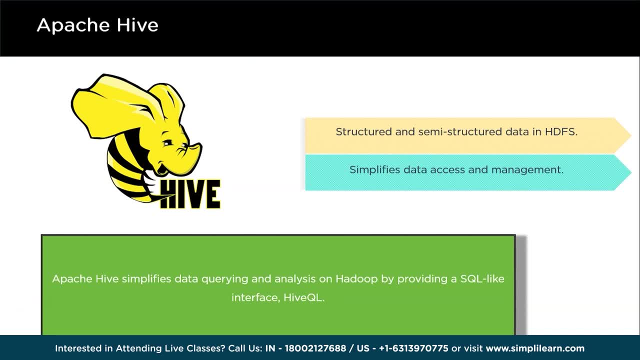 making it accessible and easy to work with. So, in a nutshell, Apache Hive is a handy tool that lets people who may not be tech-busy easily query and analyze data stored in Hadoop HDFS, Thanks to its SQLite interface and smart data processing capabilities. 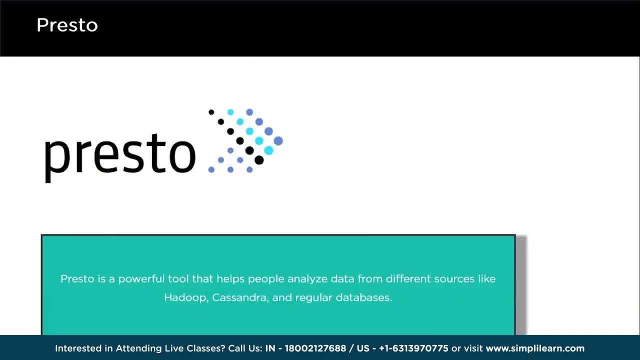 Alright, next we have is Presto. So Presto is a powerful tool that helps people analyze data from different sources like Hadoop, Cassandra and regular databases. It's like a super-smart detective that can find and make sense of data, no matter where it's stored. This is really useful. 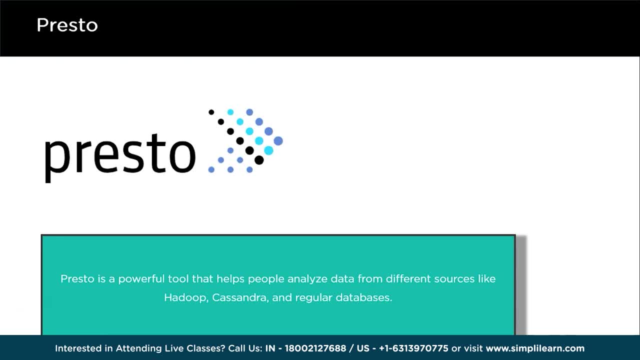 because it means you can explore and study data without having to worry about where it is kept. Imagine you have a big puzzle with pieces scattered all over the room. Presto is like the detective, who can find all those pieces of data without having to worry about where it is kept. It's like a super-smart detective who can find all those pieces of data without having to worry about where it is kept. It's like a super-smart detective who can find all those pieces of data without having to worry about where it is kept. 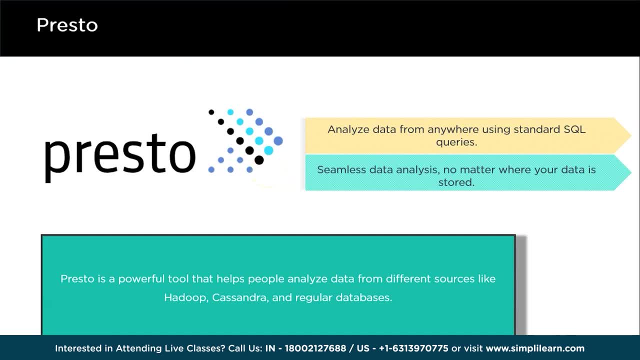 Even if some pieces are under the couch, Presto acts like a super-smart search engine for your data. It helps you find and use your data, no matter where it is hiding. So if you want to understand your business better, Presto can help you get all the answers you need from your data. So if you are 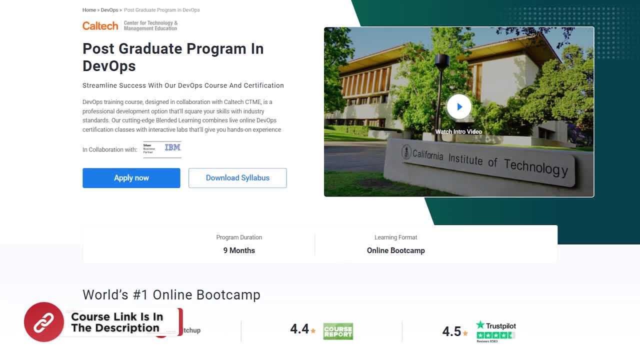 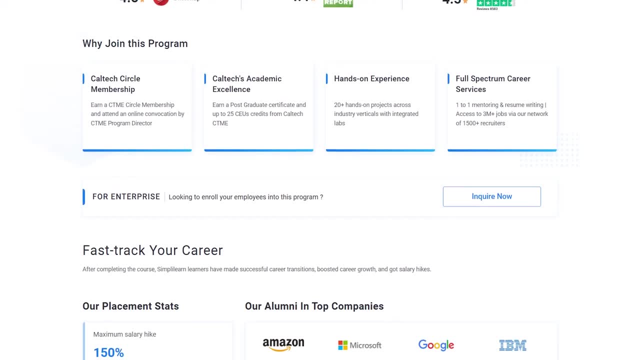 interested in mastering the world of data engineering, look no further than our post-graduate program in data engineering. This comprehensive course is tailor-made for professionals like you. In this course, you will be diving deep into essential topics such as Hadoop frameworks, Spark-based data processing, Kafka-driven data pipelines. 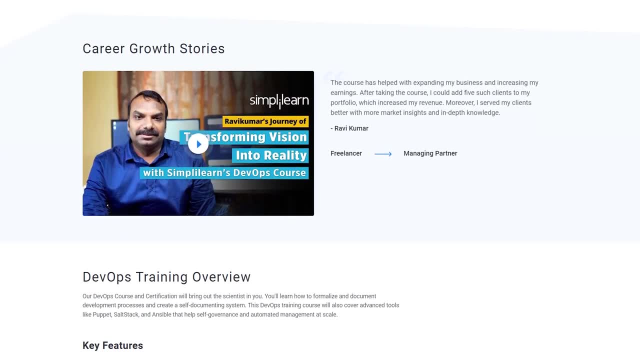 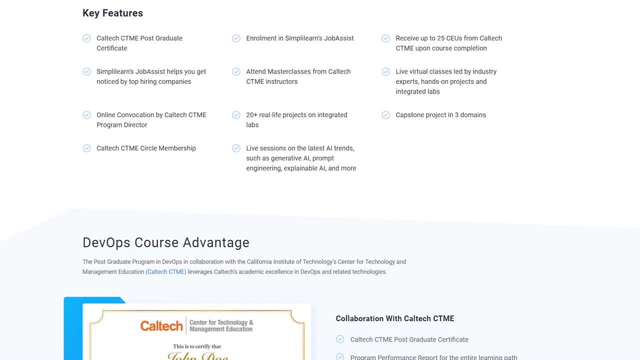 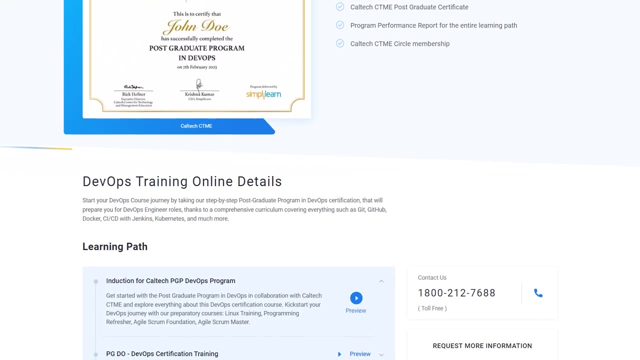 and the atrocities of managing big data on AWS and Azure cloud infrastructures. Our unique approach blends live sessions, hands-on industry projects, exciting IBM hackathons and interactive ask-me-anything sessions to provide you with the most enriching learning experience. For admission to this data engineering course, candidates need a bachelor's degree with 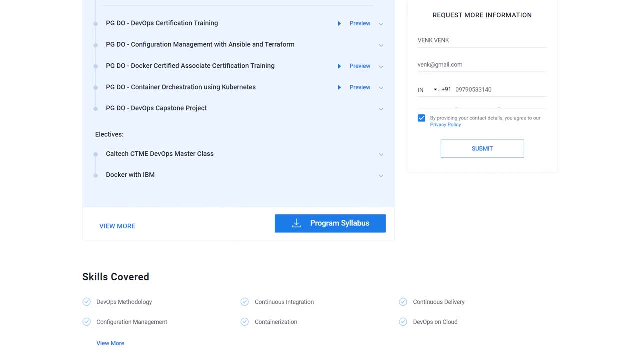 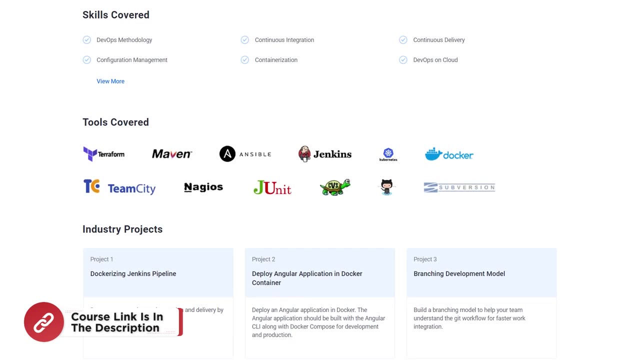 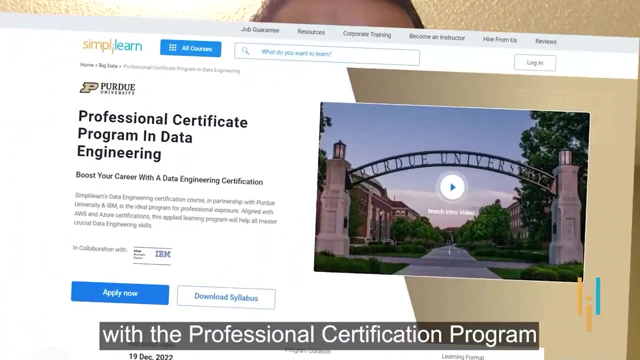 an average of 50 percent or higher marks two plus years of work experience, then basic understanding of object-oriented programming that is preferred. So elevate your data engineering skills and career prospects today and roll now. Hi, I am Asad Shah from Canada and I recently upskilled myself with the professional 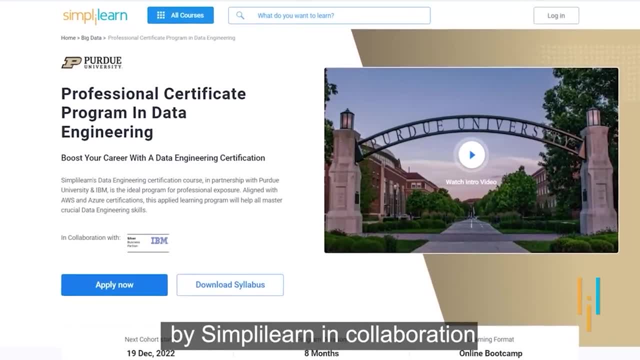 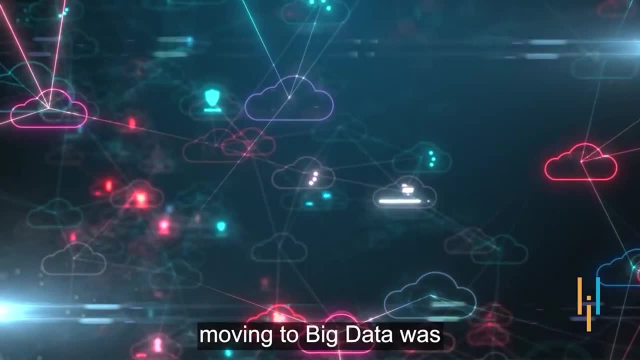 certification program in data engineering offered by Simply Learn in collaboration with Purdue University. After working for a long time in the SQL domain, moving to big data was a great challenge for me. I needed to upgrade my skills to improve my performance in my current pro course. 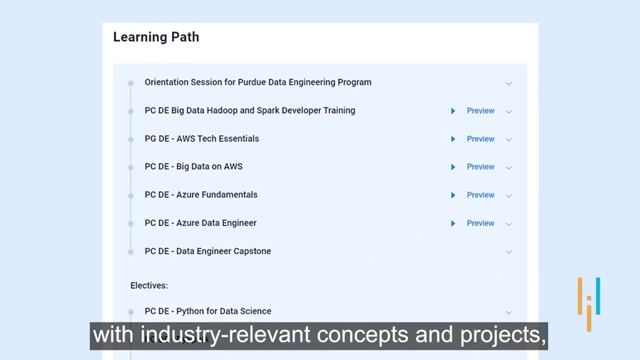 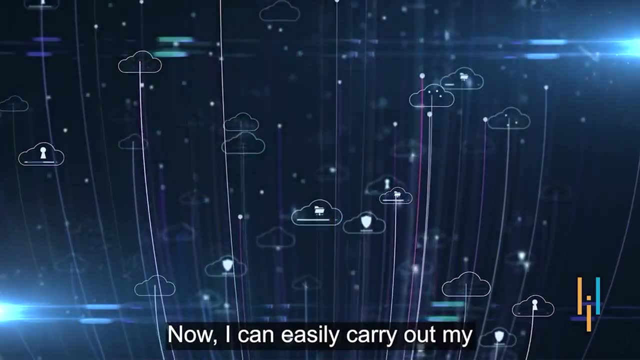 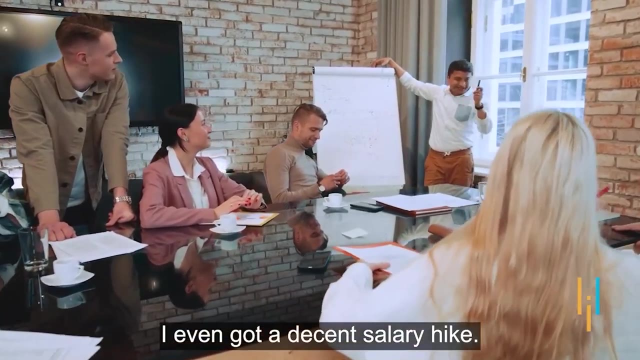 curriculum is well formulated, well industry relevant concepts and project, which helped me grasp deeper knowledge about big data. Now I can easily carry out my big data projects as well as successfully lead a team of engineers. I even got a decent salary hike. The world is moving at a much faster pace than we think. Make sure you don't lag behind. 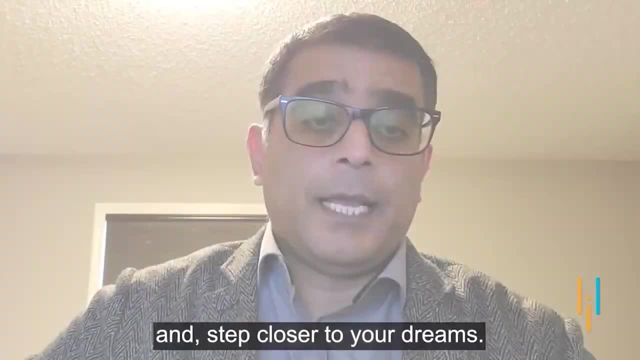 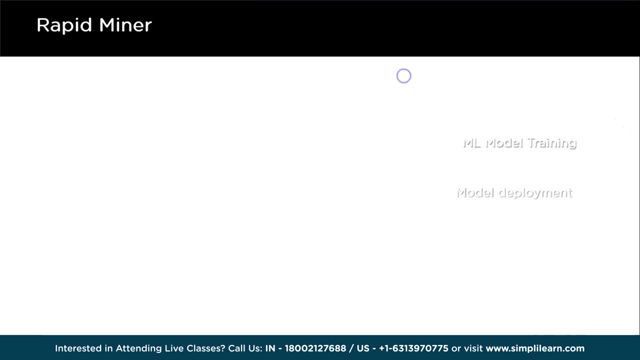 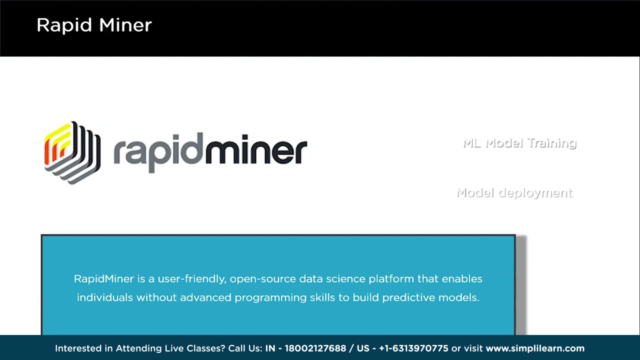 So upskill yourself and move to a step forward and step closer to your dream. Next big technology on the list for 2024 is RapidMiner. RapidMiner is a user-friendly and open-source platform for data science that helps organizations build and use predictive models, even if they don't have advanced programming skills. 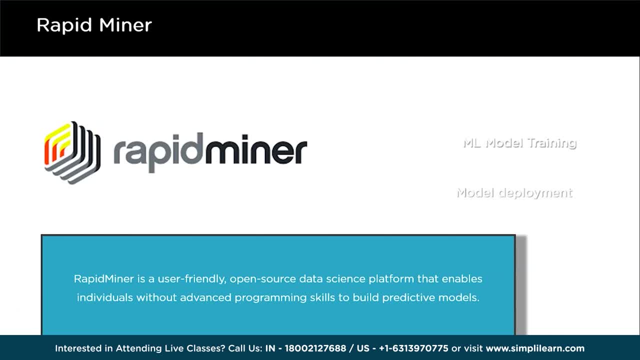 This means that anyone who works with data can benefit from its features, regardless of their level of expertise. One of the great things about RapidMiner is that it can handle a variety of tasks related to data, such as preparing and cleaning it, training it and like training machine. 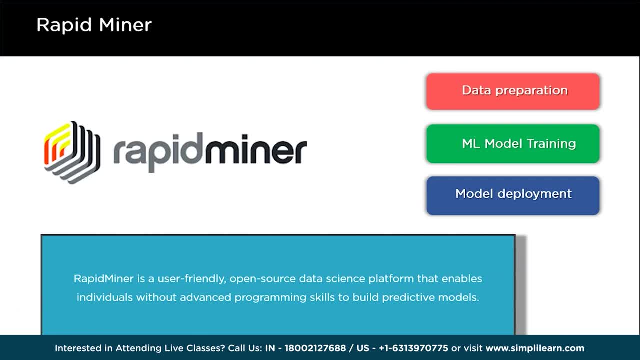 turning models and deploying these models for practical use. This makes it a versatile tool that can be used in different stages of data project. So, whether you are a data scientist or just someone who occasionally works with data, RapidMiner can simplify your workflow and make it easier to achieve your goals. It is designed to be accessible and user-friendly. 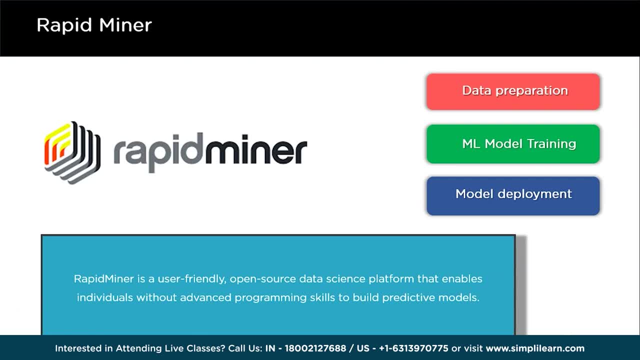 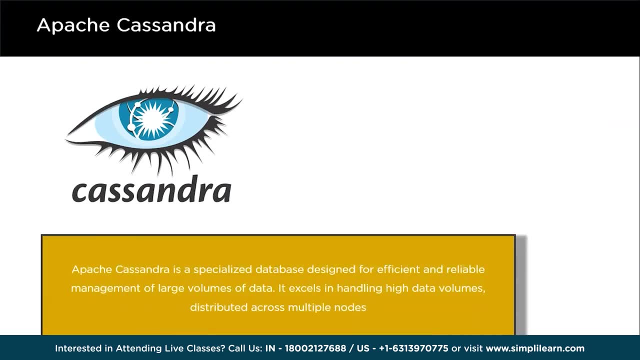 so you don't need to be a coding expert to get the most out of it. Alright, coming to the last one, that is, the last big data technology for 2024, which is Apache Cassandra. Apache Cassandra is a type of database that is. 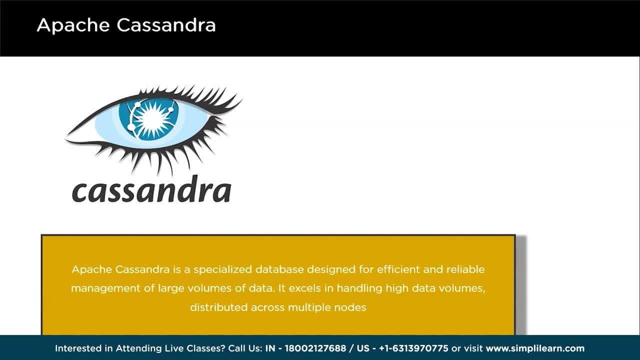 specifically designed to handle a lot of data in a highly reliable and efficient manner. It is particularly well suited for situations where you need to store and access large amounts of information quickly and without any disruptions. One of the key features of Cassandra is its ability to handle a large amount of data points across multiple computers or nodes. 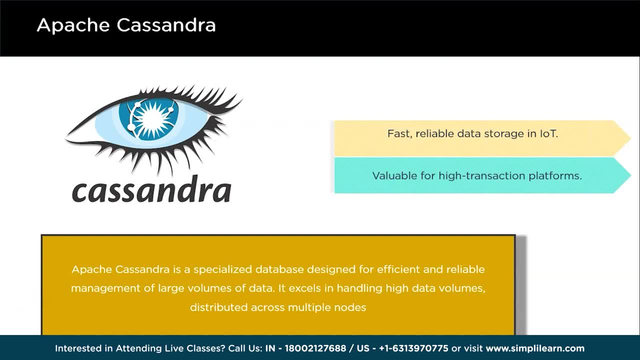 which makes it a greater choice for applications that need to process a high volume of information. This distributed nature of Cassandra also ensures that even if one node fails, the system will still keep running smoothly, making it incredibly fault tolerant. Cassandra is often used in industries.